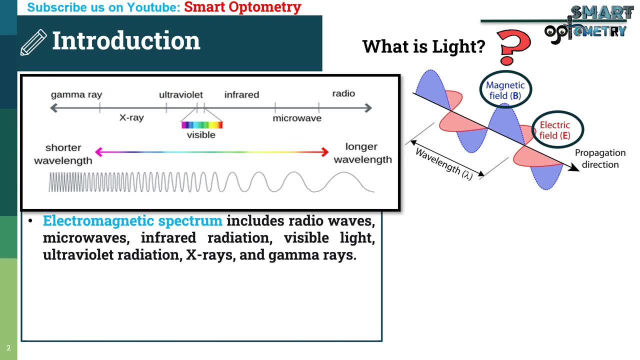 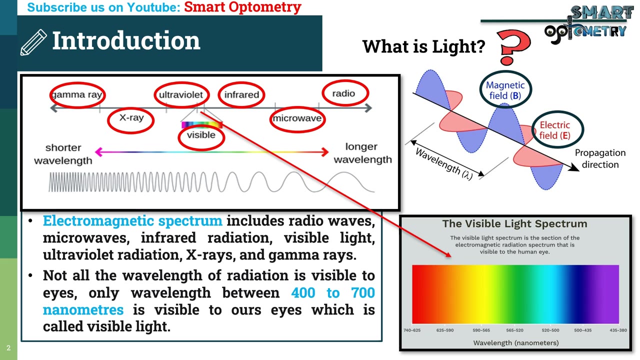 spectrum based on their wavelength. Electromagnetic spectrum includes radio waves, microwaves, infrared radiation, visible light, ultraviolet radiation, X-rays and gamma rays. Not all the wavelength of radiation is visible to human eyes. Only wavelength between 400 to 700 nanometers is visible to our eyes, which is called visible light. 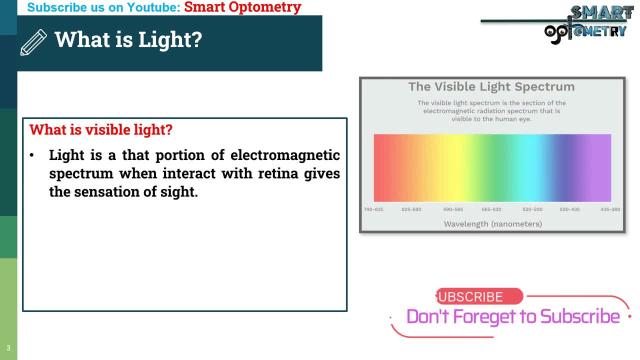 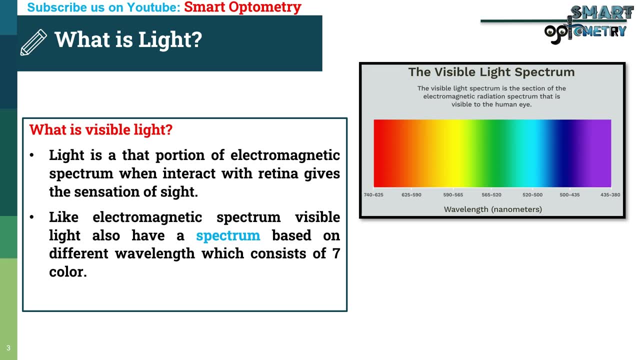 So what is visible light? So what is visible light? So what is light? Light is that portion of electromagnetic spectrum, when interact with retina, gives the sensation of sight. Like electromagnetic spectrum, visible light also have a spectrum based on different wavelength, which consists of seven color. 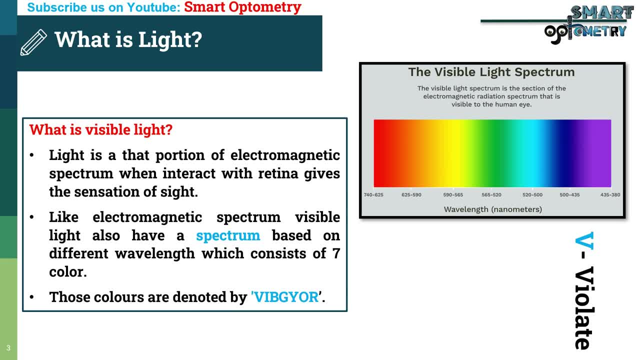 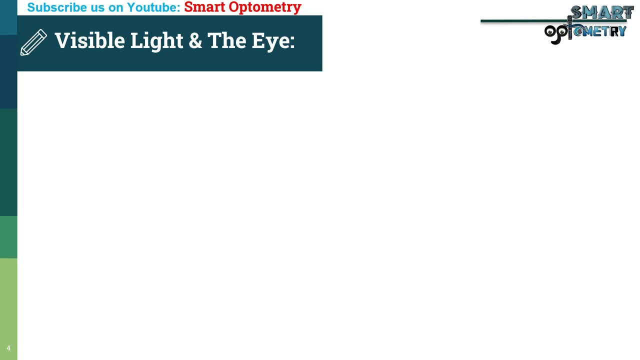 Those colors are denoted by BGR: B for violet, I for indigo, B for blue, G for green, Y for yellow, O for orange, R for red. Relationship between visual lights and the eyes. As we already know, wavelength range between 400 to 700 nanometers are visible to human eye. 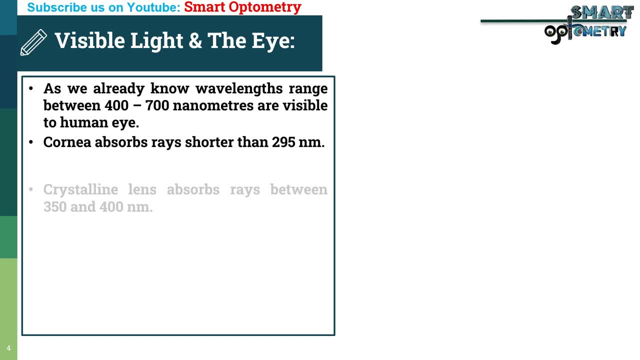 Cornea absorb rays shorter than 295 nanometer, and crystalline lens absorb rays between 350 to 400 nanometer. In aphacic eyes, the light rays between 350 to 400 nanometer can also pass on to the retina. Therefore, the aphacic eyes are sensitive. 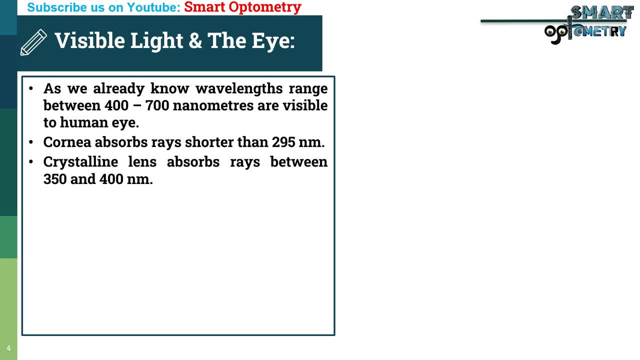 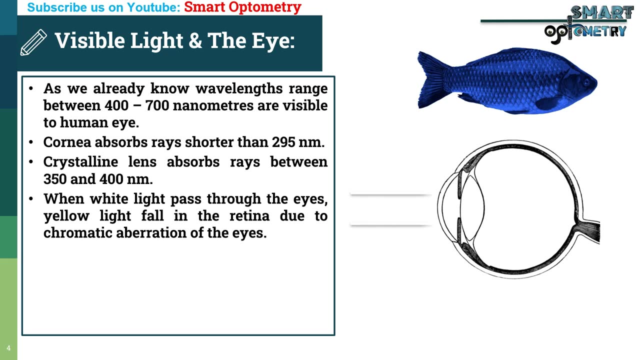 to those wavelength which gives rise to a sensation of blue or violet color. Hence the newly aphacic patients often complain that everything looks bluer than visualized before the operation. When white light pass through the eyes, yellow light fall in the retina due to chromatic aberration of the eyes. 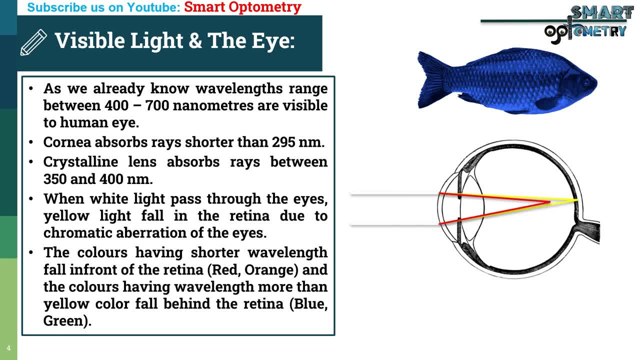 The colors having shorter wavelength fall in front of the retina, like red orange, And the colors having wavelength more than yellow color will fall behind the retina, like blue green. This principle is used in Duke room test to identify spherical endpoint during subjective diffraction.